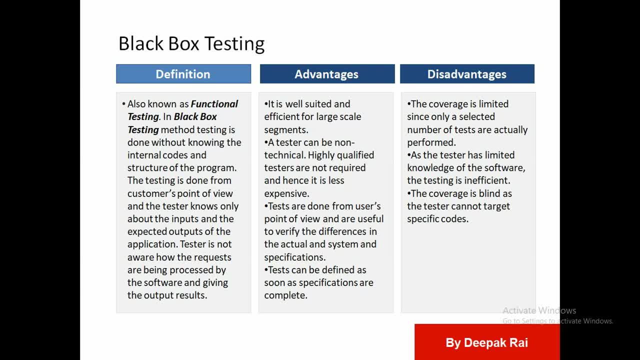 So, first of all, what is black box testing? So it is also known as a functional testing. In black box testing method, testing is done without knowing the internal codes and structure of the program. So black box testing is blind test which we don't know about the background codes of the content, Like if you are testing for the facebook. 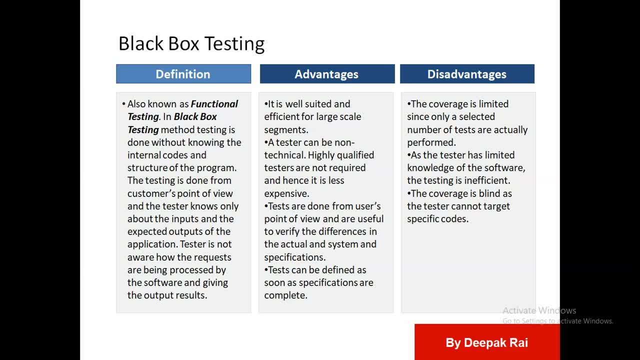 lockdown and we are working on the any specific functionality like posting the content or you can call as posting the images on their timeline. So the tester don't know about the coding part of that posting, So posting images on facebook. So without knowing any code, tester is testing whole procedure. The testing is done from customer. 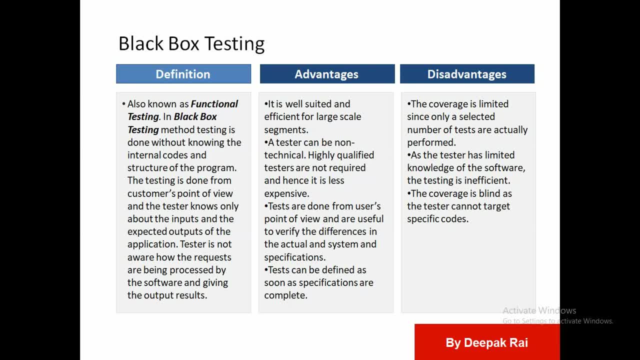 point of view and the tester knows only about the inputs and expected output of the application. So he only knows the input and output, Just like if you are entering any detail, like in login page, so login page contain inputs of the user name and password and after clicking 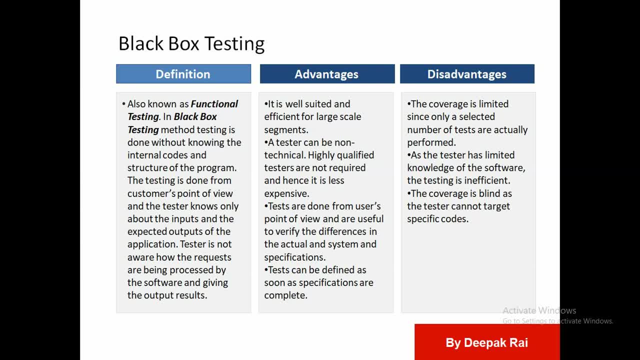 on subject. it enters into login page. so tester or customer point of view, the user who is going to test this application is don't know about their coding part, so they are just entering the input and knowing the output- what is expected output, or you can call: what is that output? 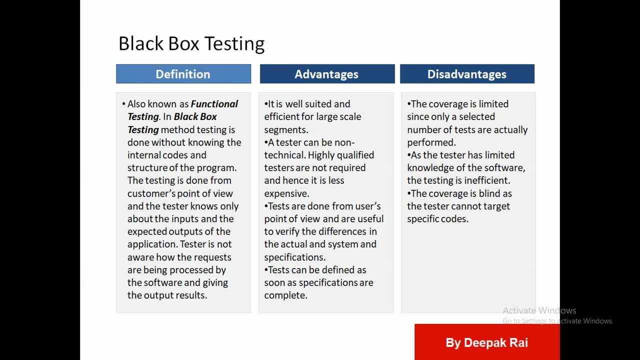 is available in their test cases or test scenarios. tester is not aware how the request are being processed by this software and giving the output to the result. that is specifically called as black box testing, as we have discussed before. like if you are working, the user is working on any facebook content, like posting the image on their timeline. so this is the. 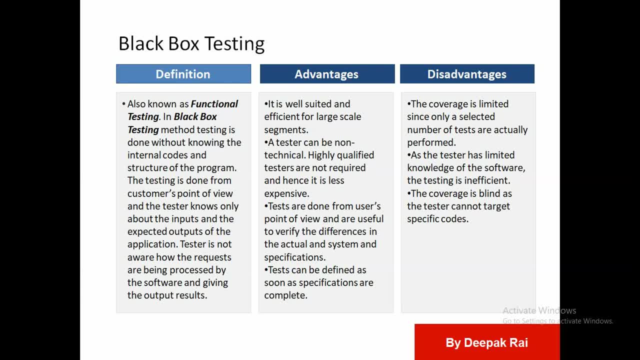 example for that, for the black box testing. without knowing any code, tester is just inserting their images and posting on their wall, or you can call as timeline. so what is advantage of the black box testing? so it is well suited and efficient for the large scale segment. then second is: 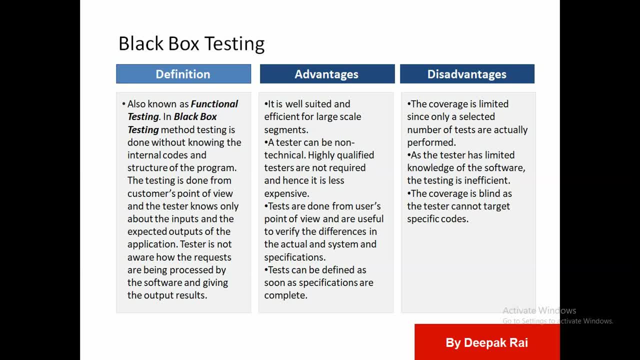 a tester can be non-technical, highly qualified tester are not required. hence it is less expensive for that without knowing code, because tester don't have to look or don't have to work on the coding part, they have just input and checking with the expected or desired result for that. 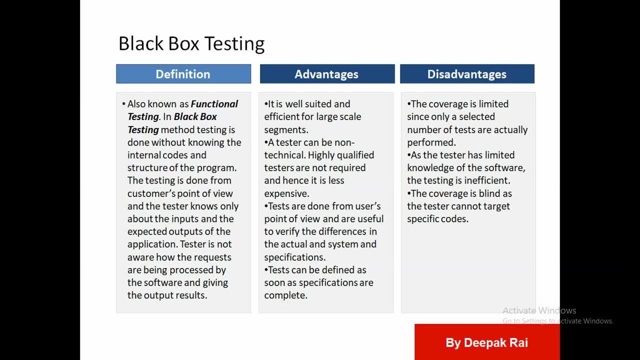 so it is not required for the high skill like engineering student or even 12th class student and also do this activity by getting input and checking with the expected output. take a look at the test results. test results: tests are done from the user point of view. that is called as it is working for the user. 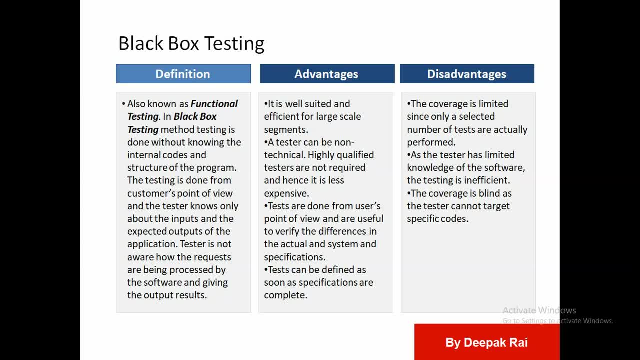 point of view and are useful to verify the differences in the actual and system specification. so what is system specification is provided by and what is the actual result? so tester is comparing that part only test can be define as soon as specification are complete. so next part is: what is this advantage of black box testing? the coverage is limited since only a 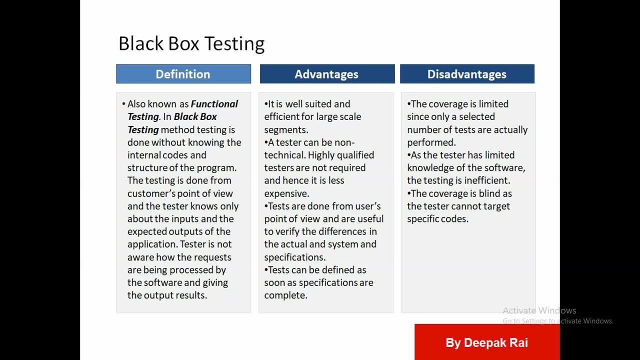 selected number of tests are actually performed, as the testers has limited knowledge of the software or coding language, the testing is inefficient because the particular tester who is doing the black box testing he don't know about the code so he is not completely testing the whole project or whole product. he is checking with the actual and expected output. the cover is blind. 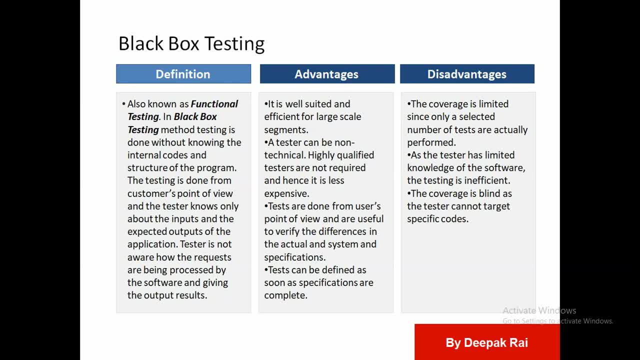 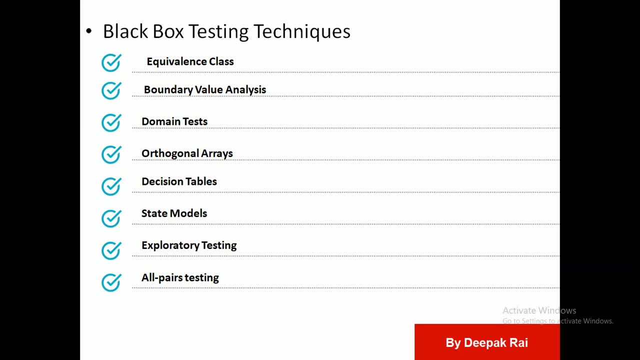 as the tester cannot target specific codes. so this is all about the black box testing. so in the next this is the black box testing techniques. by using these techniques, black box testing is performed: equivalence classes, boundary value analysis, checking each and every aspects and the side cost, or you can call as checking the boundary circles of that functionality domain test, orthogonal. 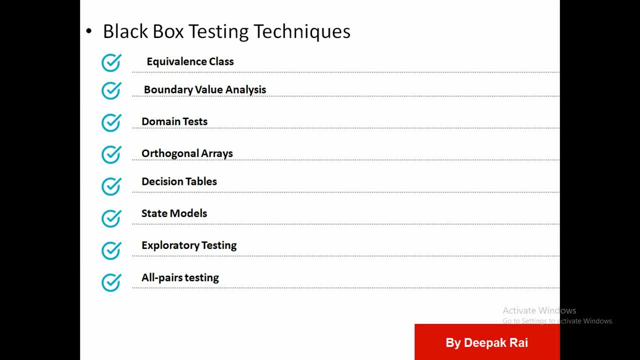 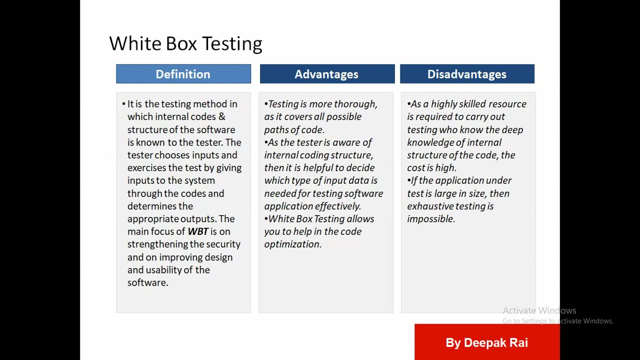 arrays, decision table, state models, exploratory testing, all pair testing. this is all our text. black box testing techniques. the next topic is for the white box testing. so it is a testing method in which internal roots and structure of the so bangs the base when you be rise to top with. but 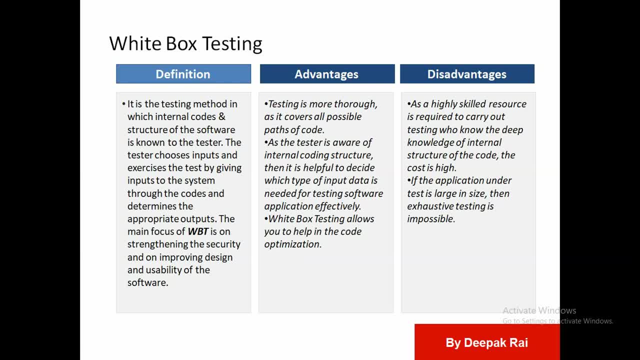 digits in this. testing methods, internal rooms, unknown with this stuff, datasER chews impotent. since i think that, be it like, even impeded the system through, this was understand it. demy name, the at the fight, the mean focus to the w would be belong to. 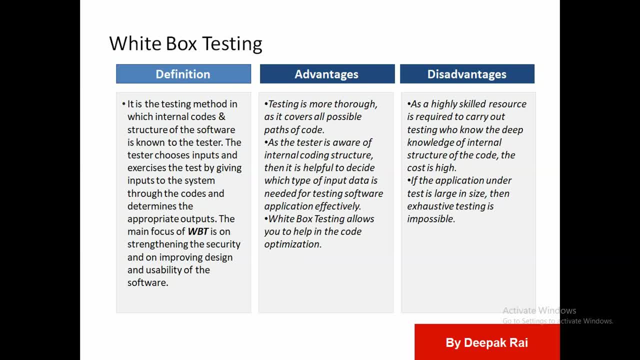 clean things, security and improving. this is a design and usability of the software. for this tester is supposed to have the knowledge of the programming language. any of the programming language is efficient. it depends on the project level. if that project is built on the C++, the tester should have the knowledge of the C++. 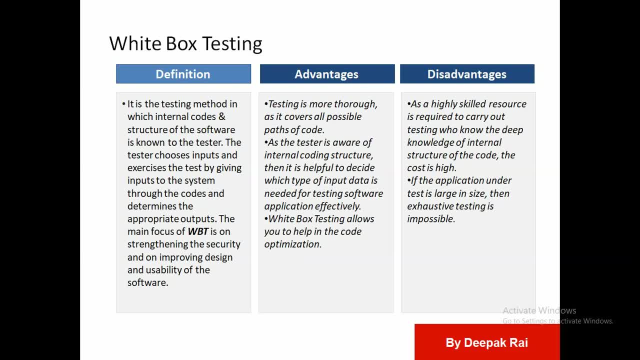 language, and if that project is created on different language, so the created language should be known to the tester. the tester should be aware of the security concerns of the project and his job is to prevent the attacks from the user and hacks which may inject malicious code into software either. 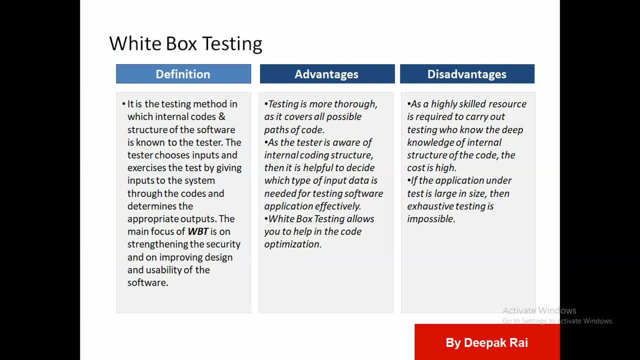 internally or intentionally or unintentionally, means the tester should be testing on the security part as well, like its availability, integrity. these type of testing should be performed in this white box: testing because the product is bug-free as well as security secure, like if I am using Facebook application and that application is not. 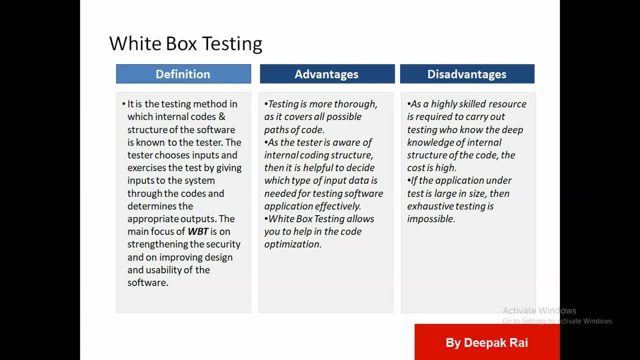 secure, or you can call that someone is stealing my details. they does like my images or my other stuffs which I stored in the Facebook post or wall, so it is unsecure application. so these type of applications are not secure because they are not secure, because they are not secure. 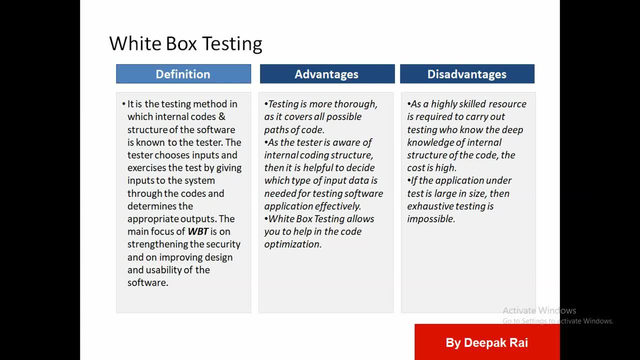 application. users should not intend to use that application, so that application is definitely should be bug-free and secure as well. so testing based on analysis of the internal structure of the component or the system is called as white box testing. so the advantage is is testing is more. 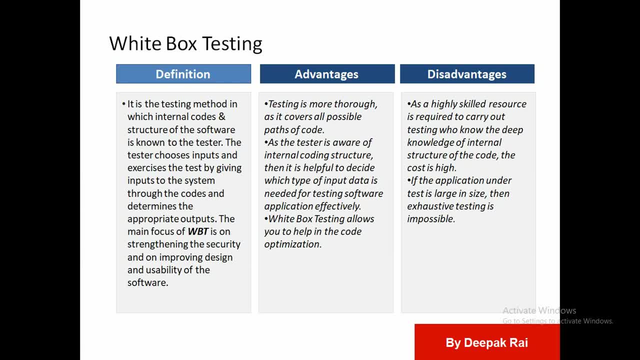 effective as it covers all parts of the code. as the tester is aware of the internal coding structure, that it is helpful to decide which type of input data is needed for testing software application effectively. white box section allows you to help in the code optimization. so next is this. 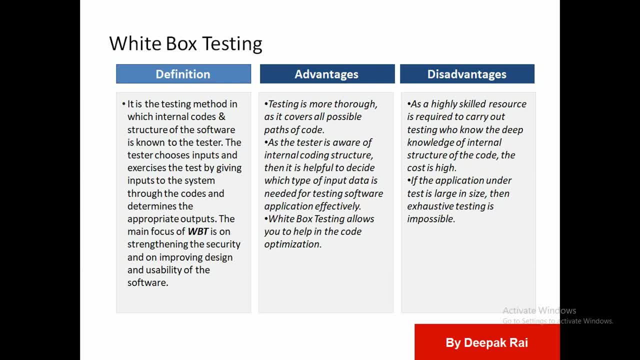 advantage of the white box testing as a highly skilled resource is required to carry out testing, so the cost should definitely going to increase as compared to black box testing. who knows the deep knowledge of the internal structure of the code? and cost is definitely going to be high if the 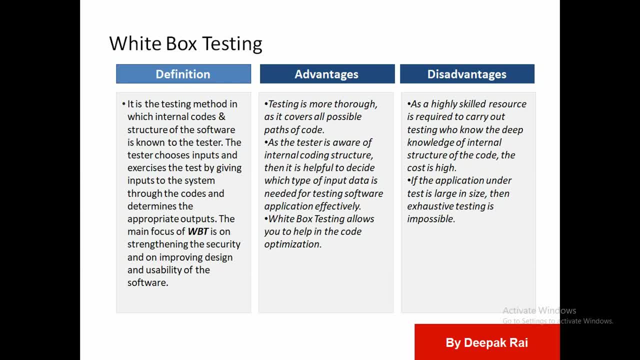 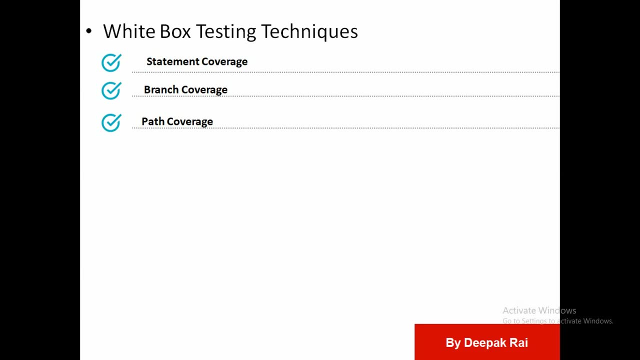 application under test is large in size, then exhaust it. testing is impossible. so what all techniques are used in the white box testing is statement coverage, branch coverage and path coverage. so basically, statement coverage, it is aimed at exercising all programming a statement with minimal tests. then branch coverage is running a series of tests ensure that all branches are. 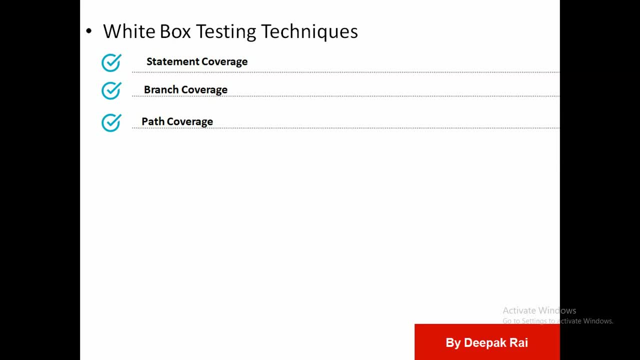 tested at least once. so if I am working in the same as we have discussed in the Facebook application, so we have to teach each and every branches like connectivity, the home pages, then contact us pages, then post pages and images, all friends. so this all should be covered and tested. 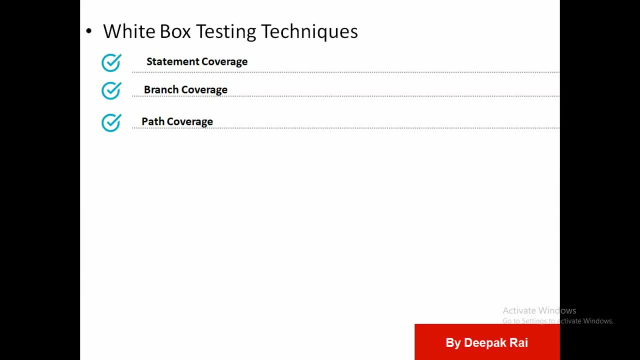 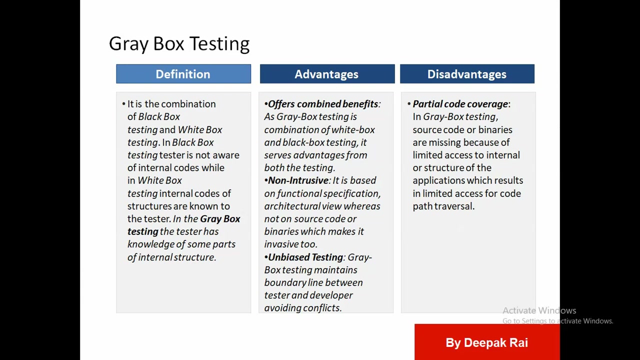 covered in branch coverage: path coverage testing, all possible path, which means that each statement and branches is covered. types of white box testing is unit testing is definitely very important part. testing each and every aspect, each and every code thoroughly is called as white box testing. next is grey box testing. it is a combination of black box testing and 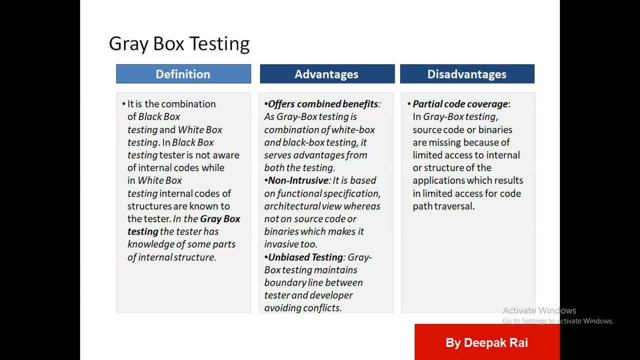 white box testing. in black box testing test is not aware of the internal codes in white box testing tester are aware of. so both the combination would be performed in the grey box testing. so that is all called as grey box testing, the grey box testing. that tester has knowledge of some parts of the internal circuit. 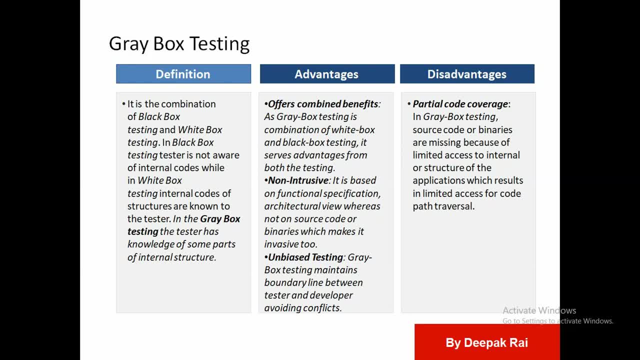 as well. this involves having access to the internal data structure and algorithm of the processes of the design, the test cases. based on this limited knowledge that test cases are designed and the tester taste the application from outside, on black box level, the brave, the gray box tester trades the. 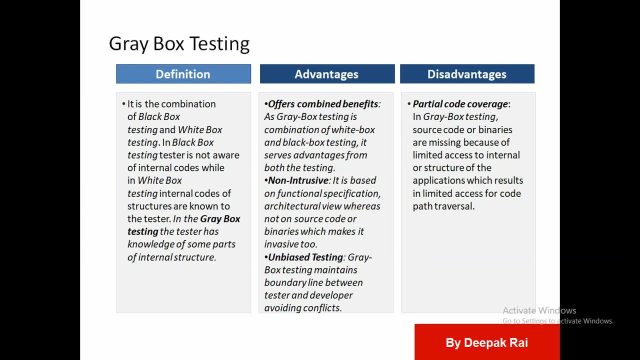 program as a black box that must be analyzed from the outside. gray box testing is considered to be not not intrusive and unbiased because it does not require that the tester to have access to the internal code. the tester may know how the system components interact or working flow, but does not. 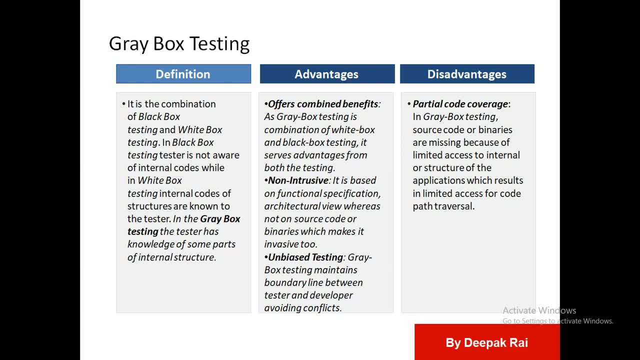 have detailed knowledge about the internal program function and operations. so what is the advantage of that? gray box testing is offers combined benefits. as a gray box testing is combination of white box and black box, it serves advantage from the both the testing methods. non-intrusive, it is based on.